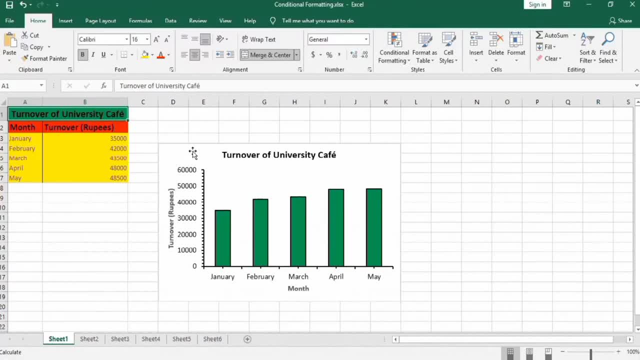 In this video, you will learn how you can change this maximum value, minimum value, major unit, which is the difference between these two data labels, which is currently 10,000, and how you can change the minor unit which is indicated by these tick marks. So let's start this tutorial. Firstly, here is the data I will 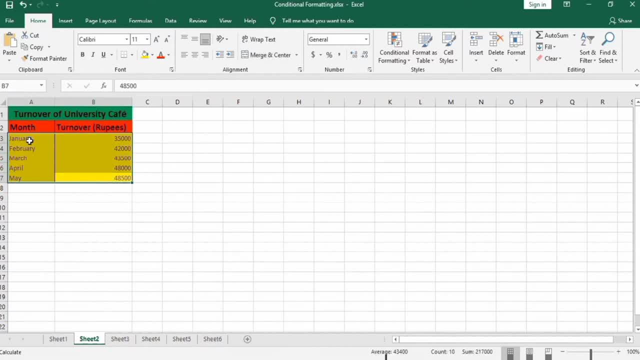 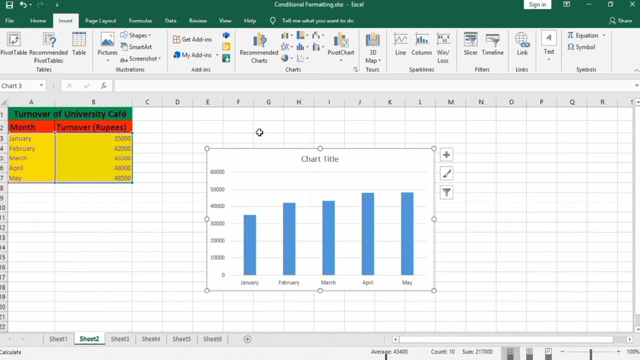 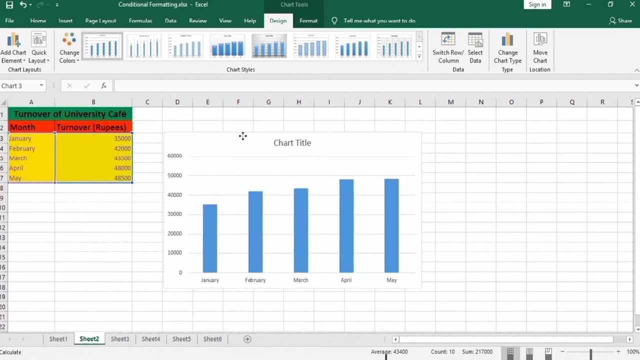 select this data, Go to insert tab and I will select this cluster column chart. The procedure is same for column chart or bar chart or line graph, so you can follow the similar procedure for all graphs. Firstly I will resize it. Now I will change these data labels. Click on this axis, y-axis. you can see it. 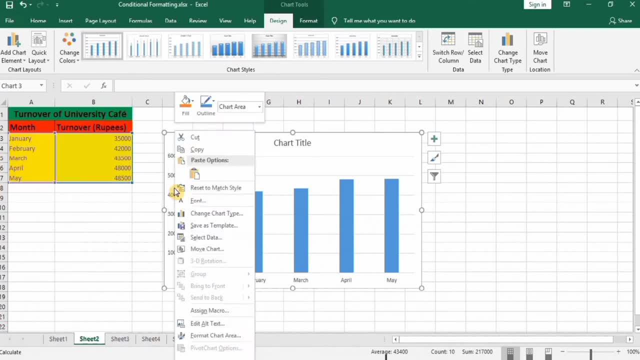 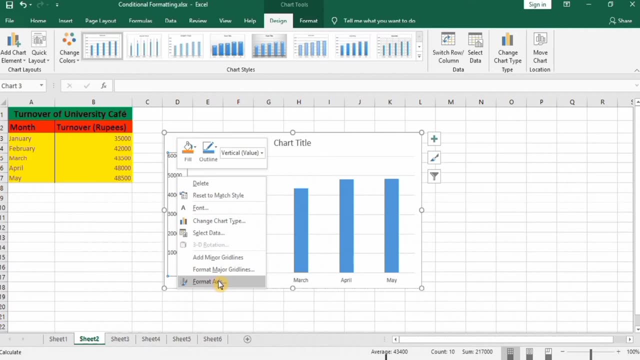 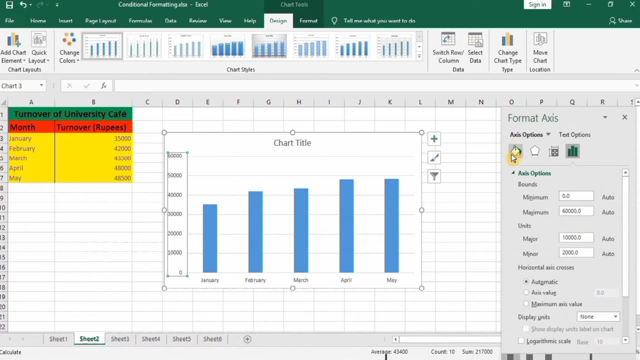 is selected now Right-click. Sorry, I will select again Right-click and here you will find the option of format axis. Click on this option and you can see here: format axis appeared here. Here different option appeared, which is field and line, effect, size and properties and axis option. Select this axis option and again. 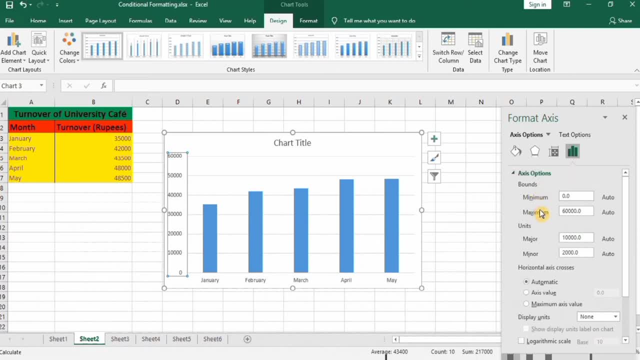 in axis option you will found minimum and maximum values. For example, currently the minimum value is 0.. I will change it to 10,000, so I will write 10,000 here. You can see here that the minimum value is now 10,000.. I. 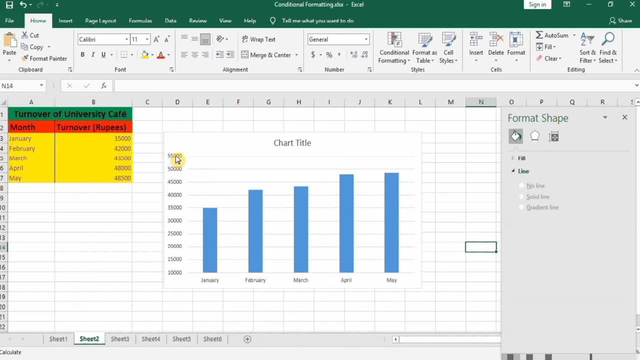 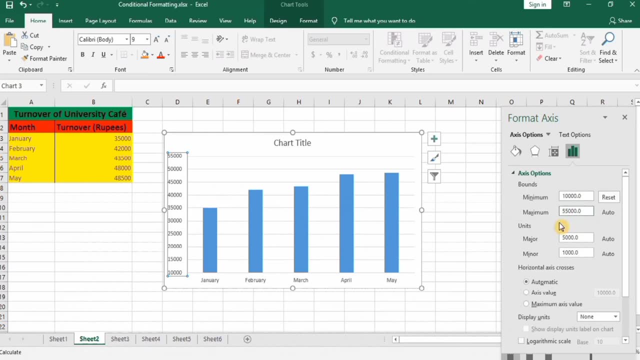 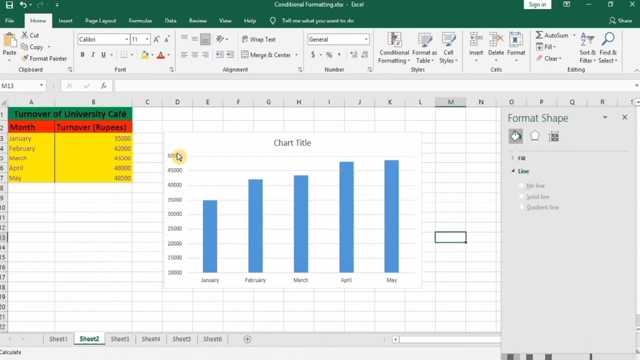 will want to change this maximum value into 50,000, so I will change it. I will write 50,000 in maximum values, So these are changed to 50,000.. Now I want to control the gap between these or the difference between these two data. 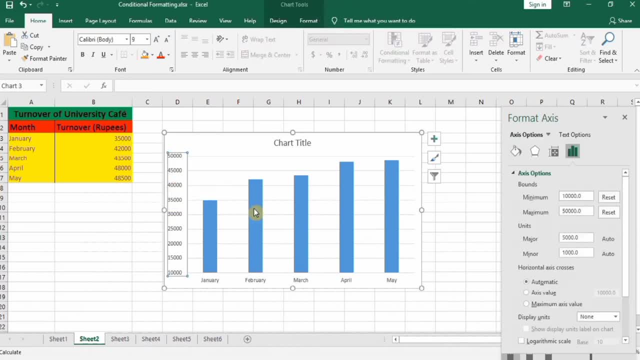 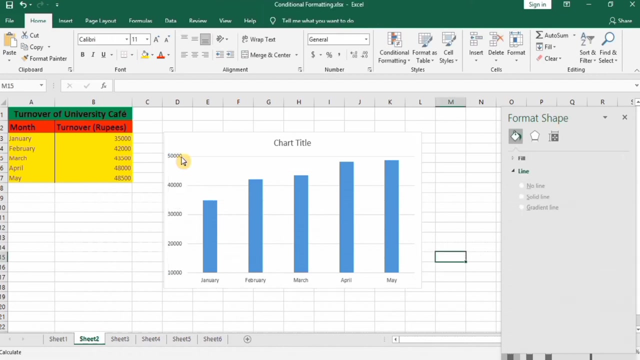 labels. Select this one and again, follow the same procedure and here, units, you will find the option of measure. I will change it to 10,000 instead of 5,000. And here you can control the minor unit. Now you can see here that the difference.